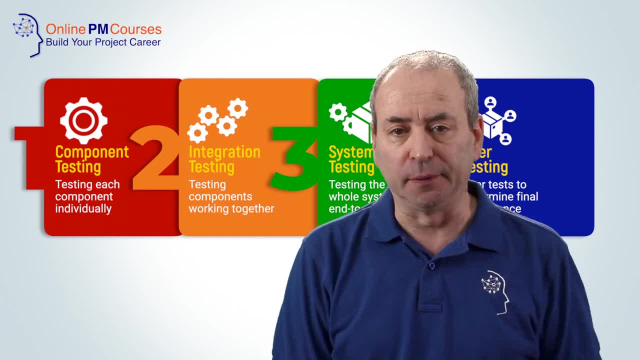 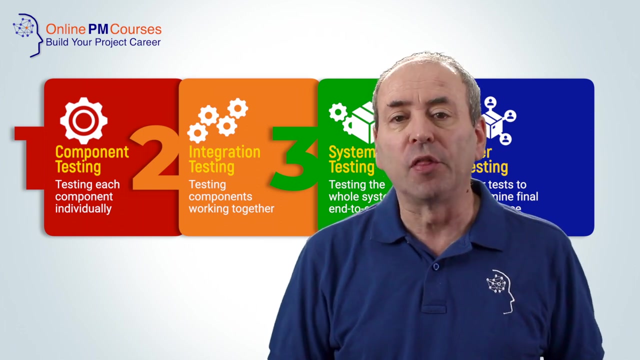 and the first is component or unit testing and, as its name suggests, this is all about testing individual components to make sure they work as designed on their own. The second type of testing is integration testing, and this is where we put components together in logical groupings or chains to make sure they continue to work as expected when connected up to other. 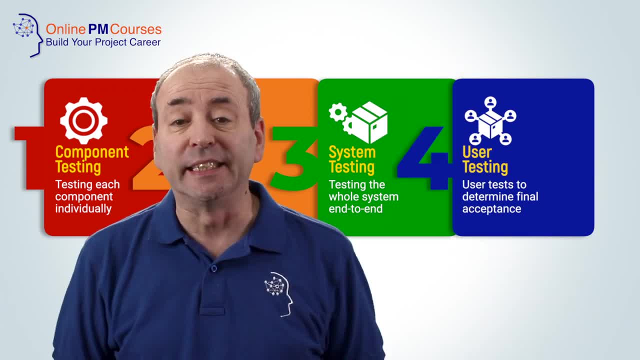 existing or new components. The third is system testing. This is when we put all of the components- the new and the pre-existing components- together to form the full system that we'll be operating and we test it to make sure the whole thing works and we can build the system and 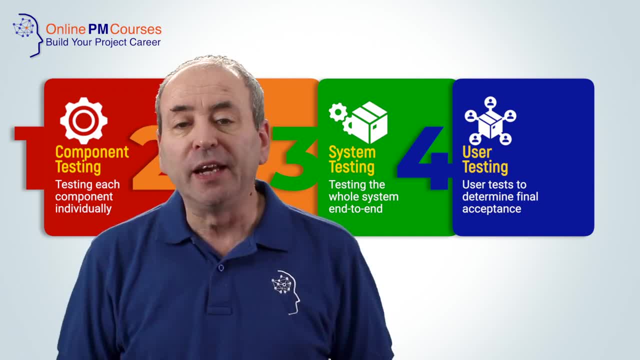 thing works properly. Finally, we have user testing, where we expose the system to the users, and the final tier of that is user acceptance testing, where our users test the system with the intention of determining whether it is usable and therefore whether they will accept it. It is the last barrier before a new system. 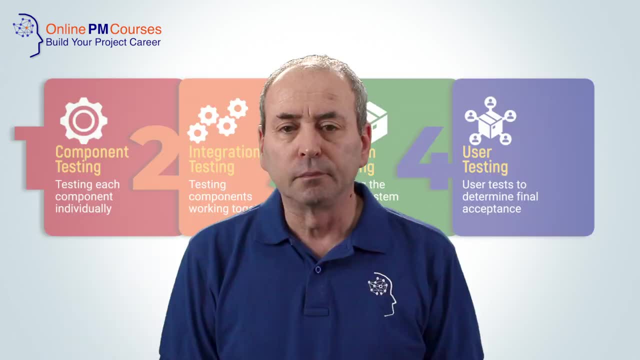 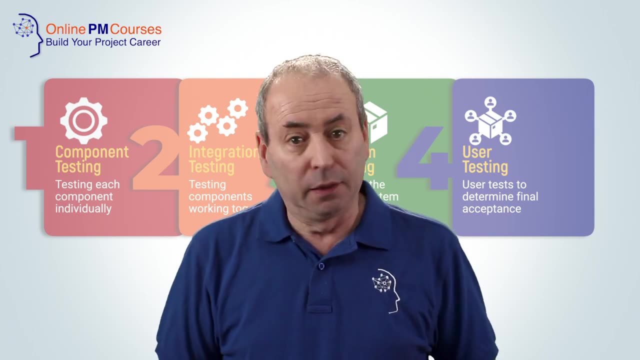 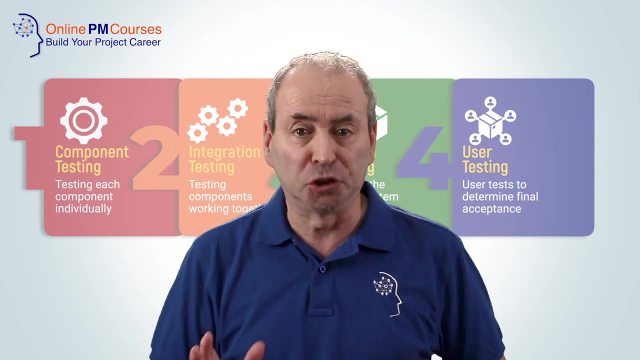 is put into live operation. The problem with testing by experts is that they tend to know how the system, the product, the software that you're creating is supposed to work, and therefore they have to work particularly hard to do stupid things. Users, on the other hand, don't know what. you're expecting them to do, so they will do what seems natural. Therefore, if you've not put in the right amount of time to test the system, then you're not properly anticipated the way that users will use the system. Users are far more likely to find the faults in your design or your implementation. 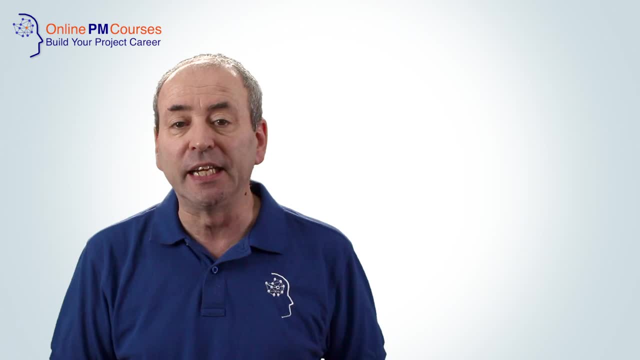 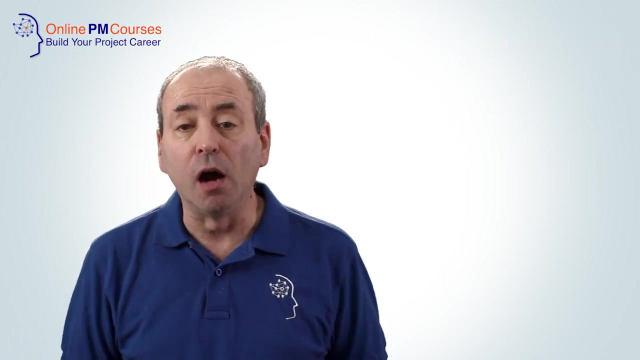 The main purpose of user acceptance testing is to validate the new software against the business requirements And of course it's the end users who are most familiar with those business requirements. So user acceptance testing is the last opportunity for your customers to test the software and to validate that it is fit for purpose. that 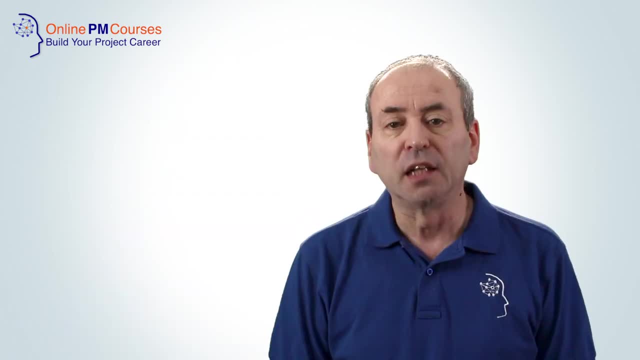 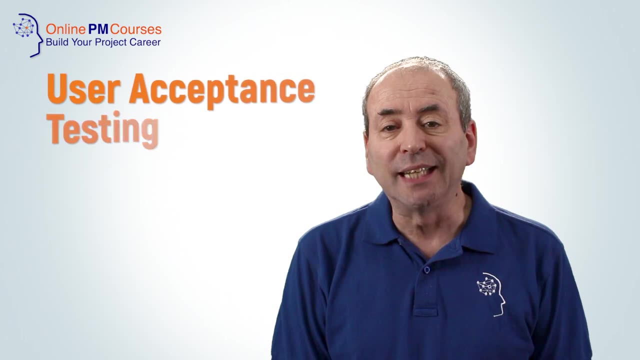 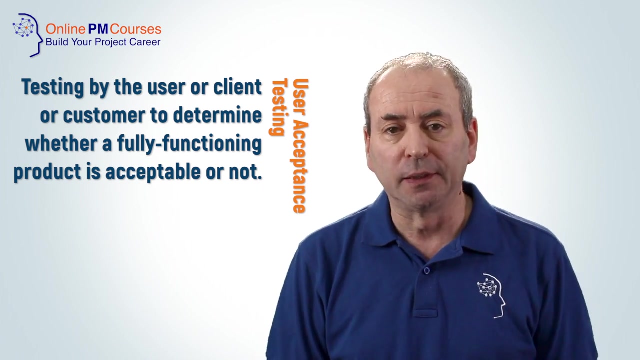 it meets the business requirements. So this gives us a working definition for user acceptance testing or end user testing. It's testing by a user or client or customer to determine whether a fully functioning product is acceptable or not. As a result, it is the lowest level of acceptance testing that you need to be able to do. 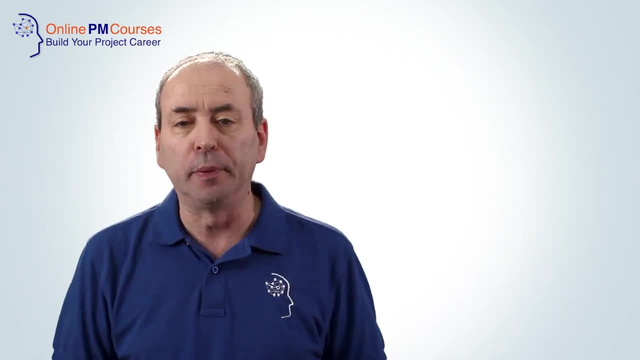 As a result, it is the lowest level of acceptance testing that you need to do. As a result, it is the lowest level of acceptance testing that you need to do. It's the last obstacle for a new piece of software to pass before it could go. 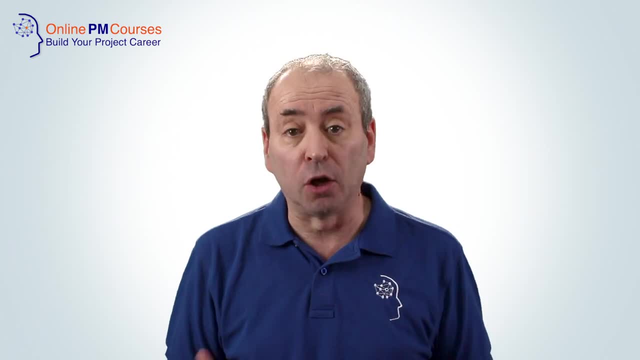 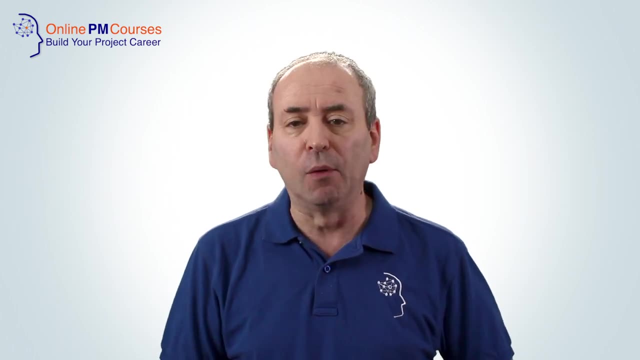 wrong. Every test manager will have her or his own detailed process or variance on the process for user acceptance testing. However, these seven steps are indicative of how user acceptance testing is carried out in a wide range of circumstances. However, these seven steps are indicative of how user acceptance testing is carried out in a wide range of circumstances. 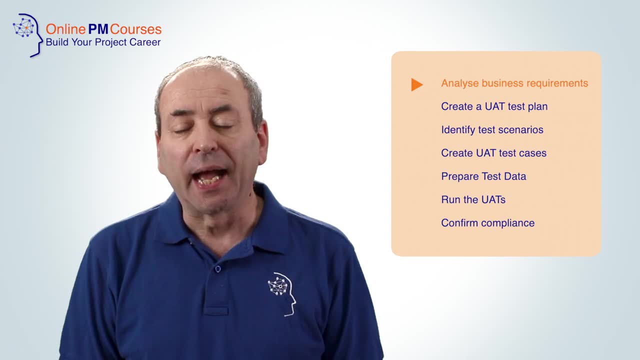 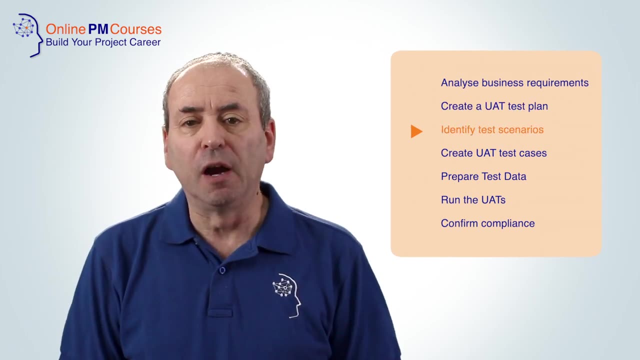 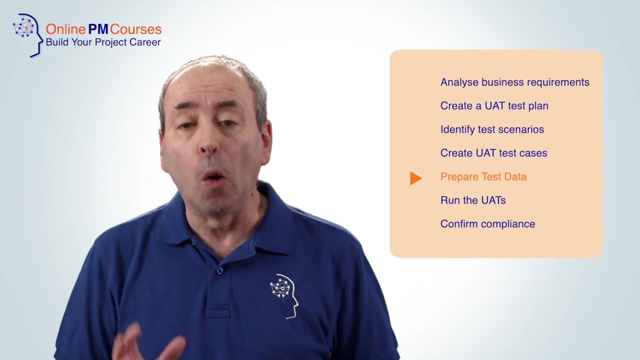 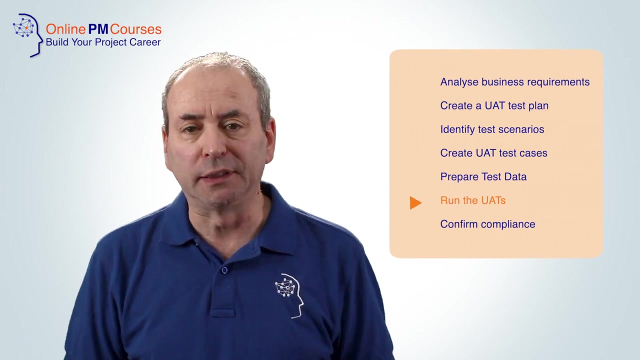 First, we analyze the business requirements and second, we create a user acceptance test plan. then we identify realistic test scenarios and then, fourth, from these we create the user acceptance test test cases. then we need to prepare test data that as closely as possible mimics real-life production data. step six is where we run the user acceptance tests. 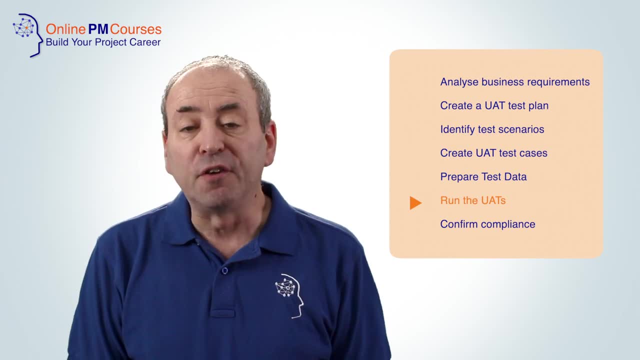 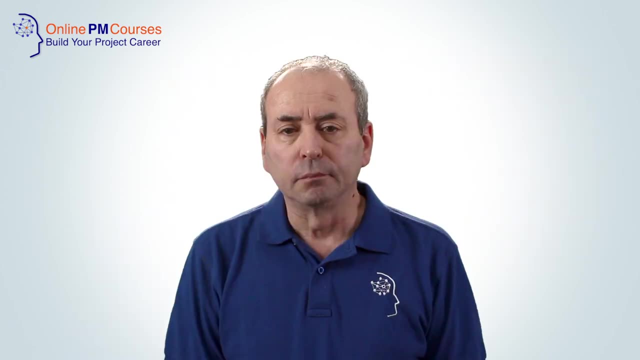 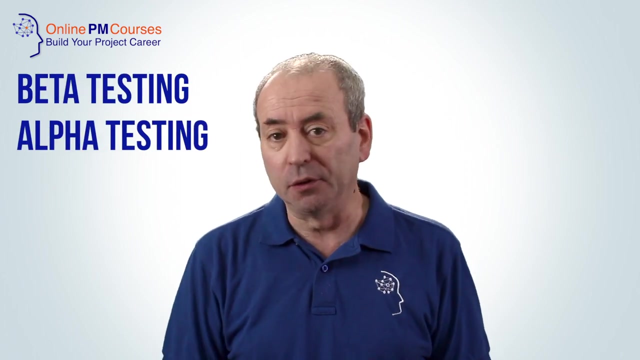 and record the results and finally, at step 7, we confirm the compliance with the business requirements. now many non specialists will have heard the term beta testing and possibly alpha testing too, and even if you've never heard of alpha testing, the very existence of beta testing suggests there. 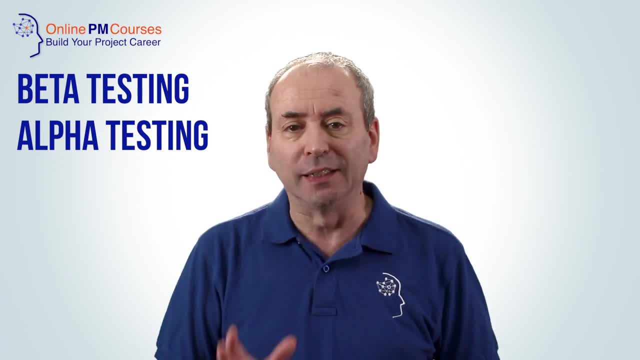 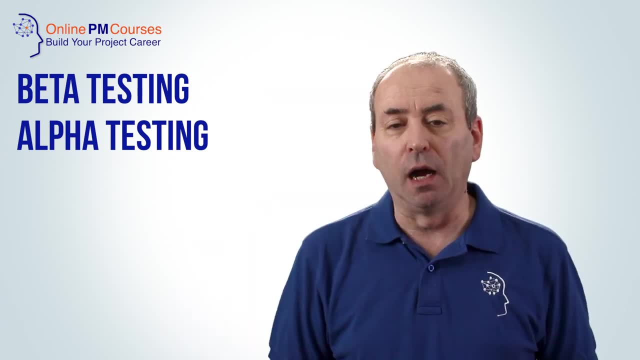 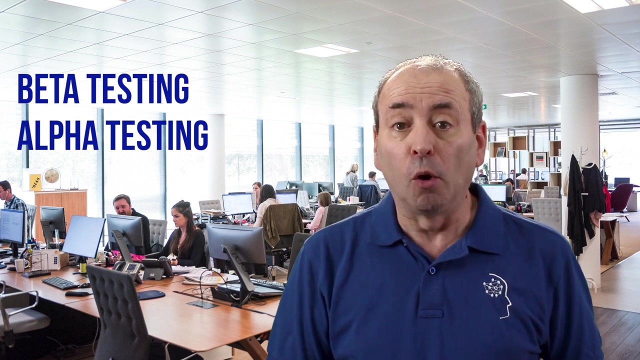 must be an alpha test. so how do alpha and beta testing differ from one another and from user acceptance tests tests? alpha and beta testing are primarily about rooting out the very last bugs in a tested software product. they do this in a real user environment to give the development team the closest possible understanding of how their 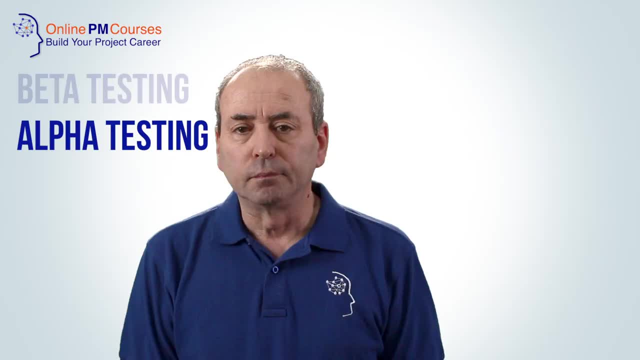 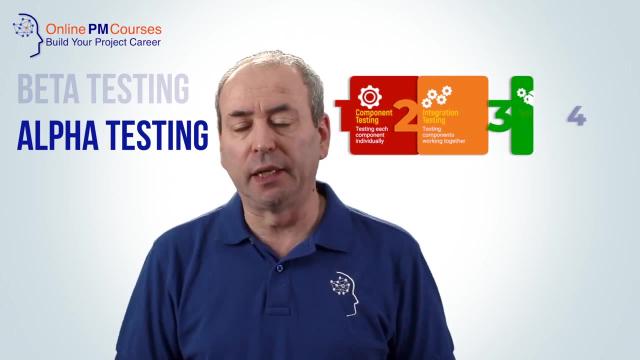 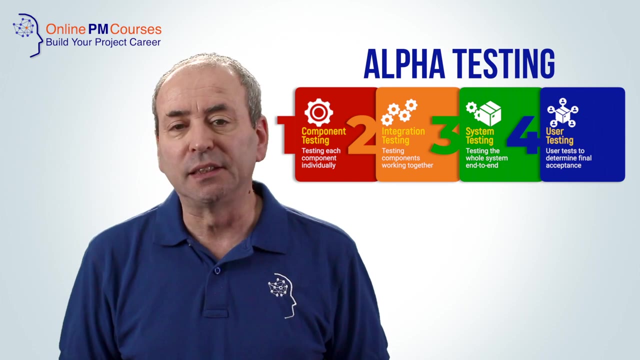 software will perform in the real world. alpha testing is a form of internal acceptance testing. it can either be the final stage of a system test or the first stage of a user test. in the first case, where alpha testing is the last part of systems testing, it's usually carried out. by the software quality assurance or testing teams. they're looking for the final bugs that they can remove before exposing it to real users. however, alpha testing can also be done by real users in a real situation. however, when real users find bugs in an alpha testing context, then they will be.